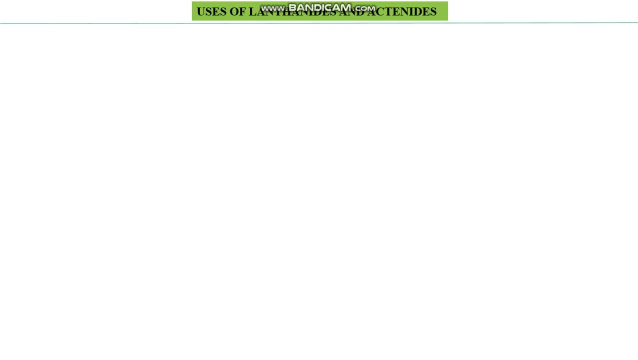 uses, because we discussed some in your previous lectures. for example, in nuclear reactions they were used as starting materials for production of energy. so that can be one of the fantastic use of these metals. let come to the point that. how many other uses of lanthanides and actinides? 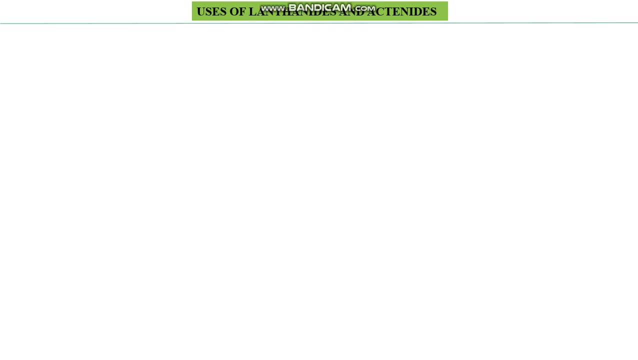 do have in everyday life. so the first one is they are used in the production of pyrophoric alloys and if you go to definition of pyrophoric materials, so pyrophoric materials are those materials. when they come in contact with air within five minutes they catch fire. also, sometimes they can be defined that they are those materials. 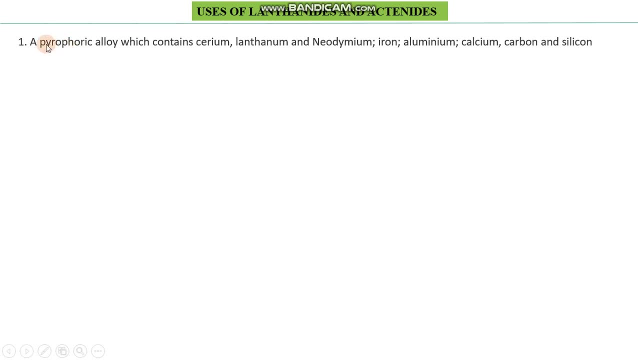 which catch fire above 50 degrees c. so those materials which catch fire either above 50 degrees c are they come in contact with air or oxygen and catches fire. so they are called pyrophoric alloys. so an alloy, definitely you are aware of alloy, that this is a mixture of two or 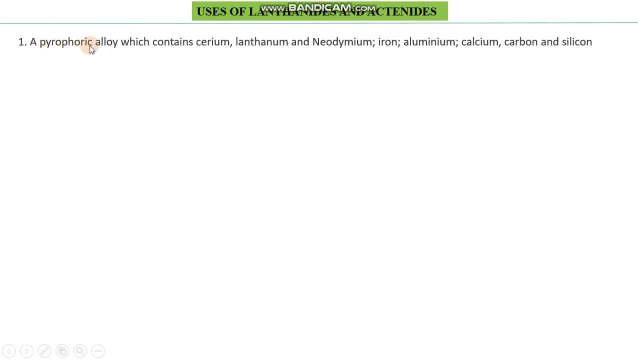 more than two metal species so pyrophoric alloys are formed are. the lanthanides and actinides are integral part of pyrophoric alloys. they contain cerium, lanthanum, neodymium and some non lanthanides and actinides metals, for example iron, aluminium, calcium, carbon and silicon. so these are the alloys. 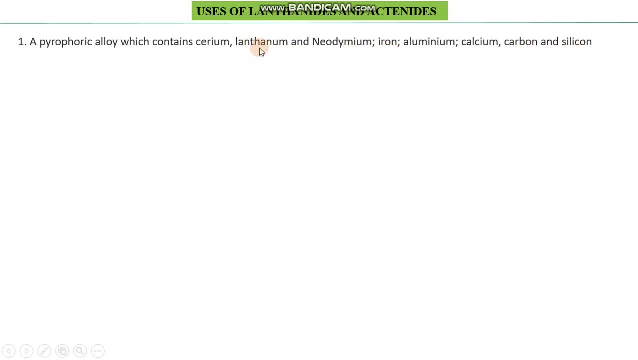 so whenever these alloys come in contact with air, they catch fire are whenever their temperature is raised to raise above 50 degrees c, then they catch fire and therefore they can be used for certain purposes which we are coming to discuss. on the basis of this nature, the pyrophoric alloy is used in cigarette lighters and i think there is a very recognizable 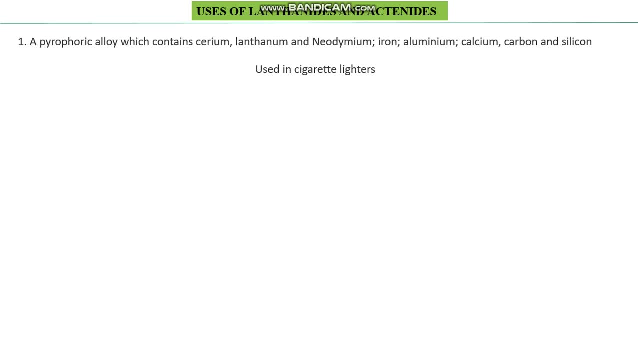 point to highlight so that i should mention also you can see, for example, in this video of the video, one of the further references it is found in the haswell related, perfectly think there is no need to explain further the cigarette lighter that what is inside and how it catches fire, or how it is used for firing purposes or in. 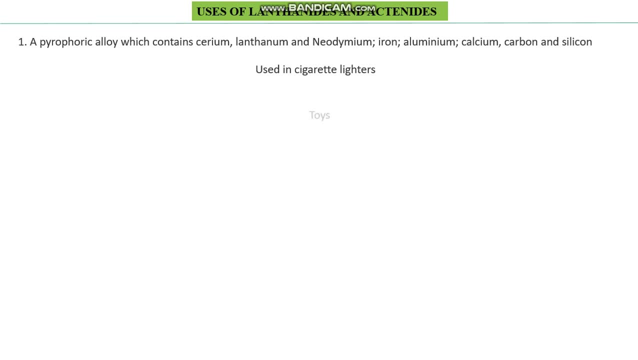 order to ignite something. they can also be used in toys and in flame throwing tanks. so this is related to defense and in this case, such material or this pyrophoric alloy is used in order to throw flame against someone. so for use, for our use, adverse purposes, adverse effects. they can also be used as in: 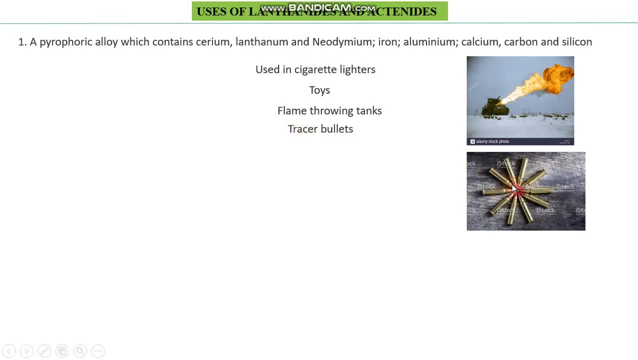 tracer bullets. there are two types of bullets, one type of bullets. they are given here in this figure and probably you are aware of bullets and I am sure that each of one have bullet at your home. let us- your parents are your elders at home- that what type of bullets are you using and what type of bullets are you? 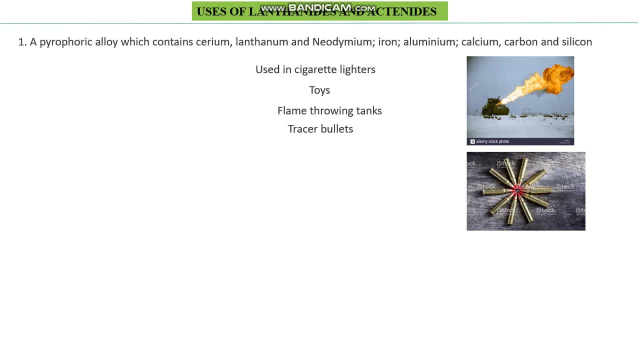 using and what type of tracer bullets are these bullets are? normally they are fired at the occasion of happiness in our areas or in our societies, and they can be seen from far away whenever they are fired in the during night time. so these are special bullets which are fired during night time, not during day. 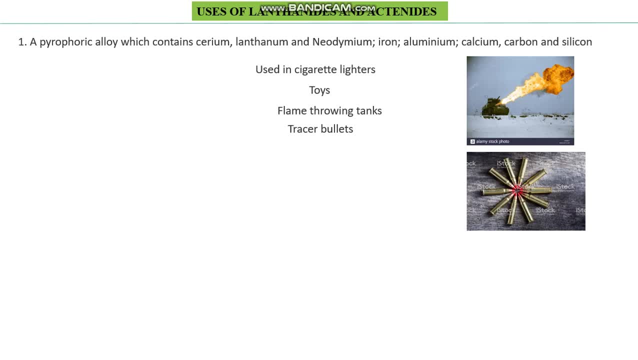 times and we can see that how far the bullet is. it's traveling in the air and one can enjoy it. so in tracer bullets they can also be used. another use of lengthen eyes and actinides is the use of Syria and Torea. they are used. 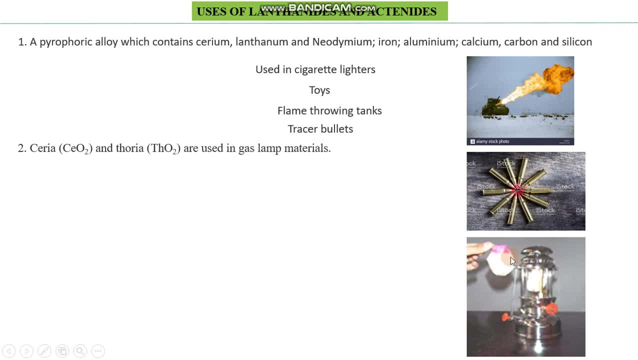 in gas lamps, in case lamps, this is the gas mantle, and gas mantle is used normally in gas cylinders or something like that, which is used for lightening purposes only, not for cooking purpose. so whenever normal or ordinary gas is used, it is ignited, so the light comes from the ignition of normal gas. this is not enough, but 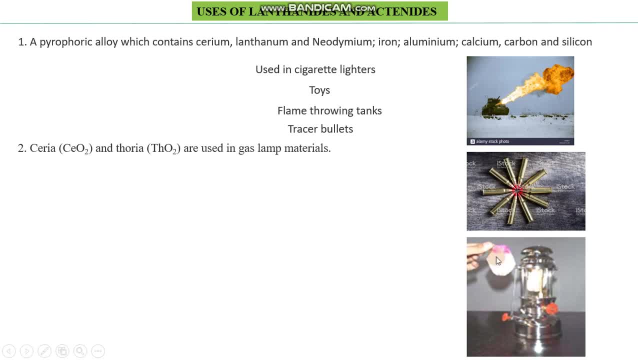 whenever this mantle is used so it produces more light and therefore it is used during the time of load shedding, for example. in our area are in those areas where there is no electricity, so the gas mantles or gas cylinders for lighting, for process, can be used normally. this, the use of this, these 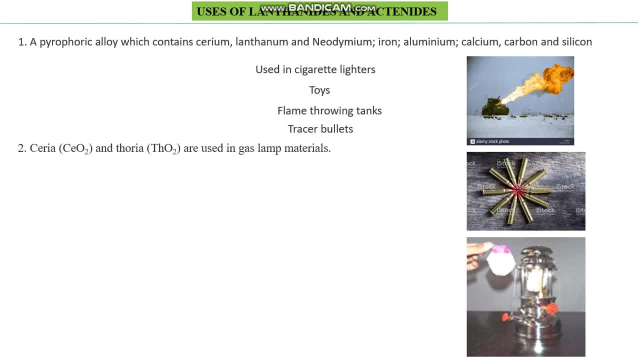 cases is becoming less and less in our society due to the electricity or which is commonly used in our areas or houses, or homes or emergency lights are now coming. they are electric, they are rechargeable, so they are more economic. so therefore, we are using the emergency lights nowadays at homes, but 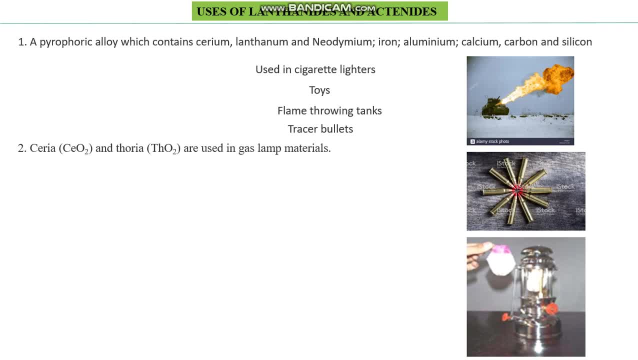 if you ask somebody. so in market I guess mantles are still available and I am sure everywhere they will be accessible. cerium salts: they can be used in drying, in dying of cottons, to to color cotton, to dye cottons. so some industrial process would be involved and cerium salts are used there in cotton industry. 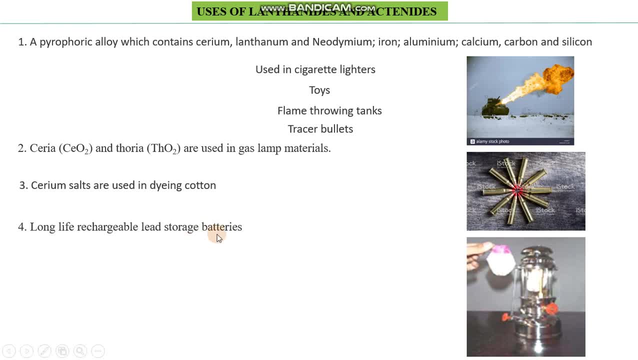 long life rechargeable lead batteries, which is actually used for storage of energies. so they are also formed of lanthanides and actinides, or lanthanides and actinides. they are used in the production of rechargeable batteries somewhere then, as you are aware of the compounds of lanthanides. 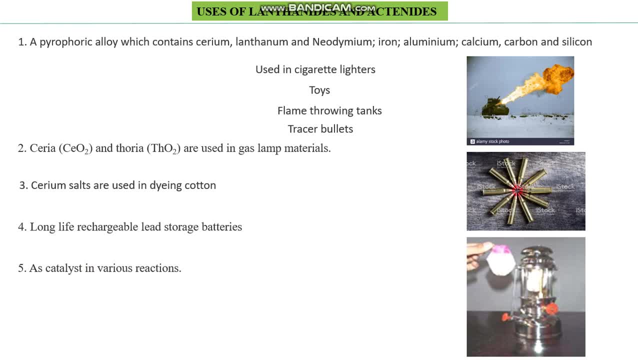 majority of lanthanides and a few actinides, so their compounds are available and these compounds are used as catalyst in order to give various products which are commercially, are industrially important. so their compounds can be used as catalysts and the the use of catalyst is normally this: 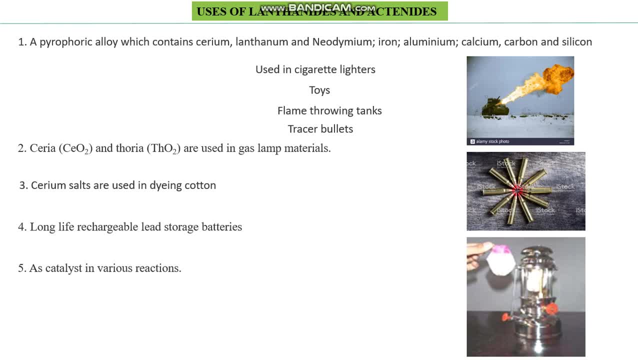 is stored. green environment are green chemistry, in order to eliminate toxic things like solvents and other chemicals and to carry out reaction at low temperature in the presence of least resources. then lanthanides and actinides: they are used in metal alter Brauna's. we are coming to our metal illmic reactions there toward. 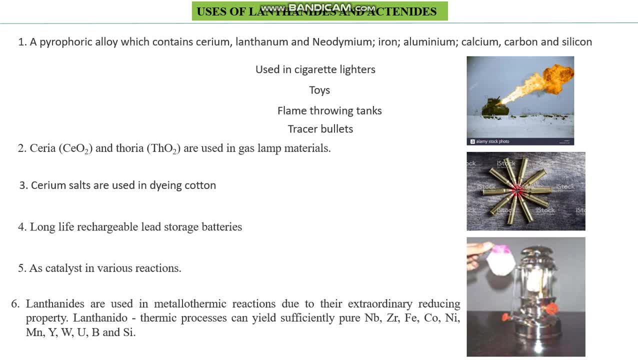 metal illmic reactions are and these metal illmic reactions, definitely metal, is very different. video in the prescription of at the first Что как recordings of metals and the research that shows a lot if the find the source materials of this leaf and you see that. 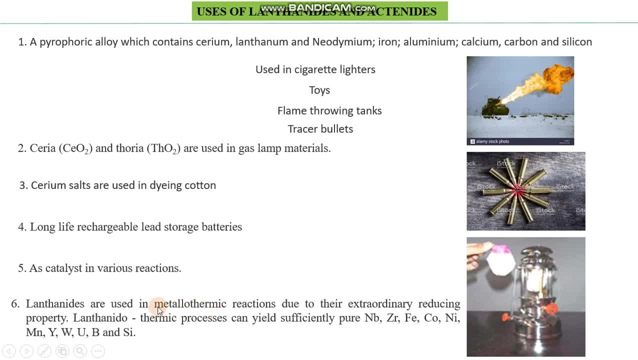 the binomial nomenclature, so metal and thermic. so the energy is produced because of use of metal. so in these reactions metals are used and due to the use of metal a certain amount of energy would be produced, and that amount of energy will be used for useful purposes. now, this why they are. 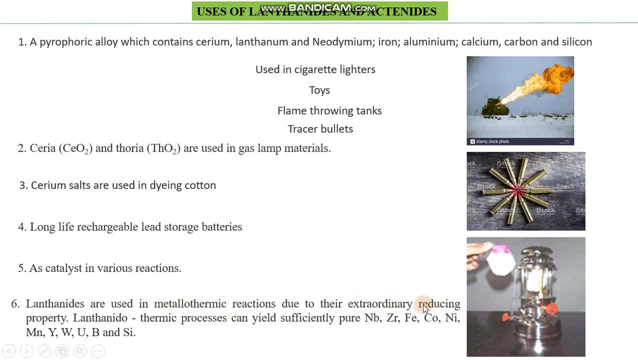 used in metallothermic reactions. so we have already discussed the reducing power of lanthanides and actinides, since they possess extraordinary reducing power. on the basis of this good or more reducing power, we can say they can be used in metallothermic reactions and these metallothermic 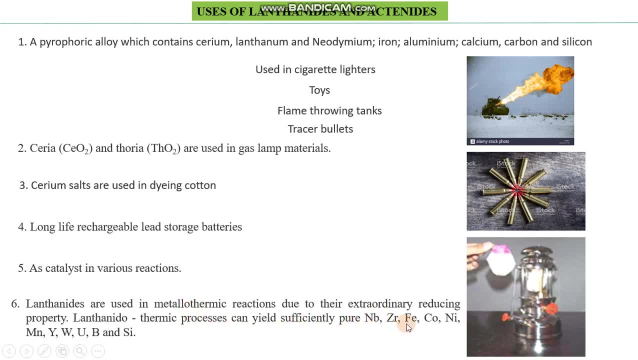 reactions, for instance, are used to obtain metals in power form, so these metals can be lanthanides and actinides themselves, or can be other metals than lanthanides and actinides. so these are some examples of a Iraltaic reaction that niobium in power farms are coonium, iron, cobalt, nickel, manganese, yttrium. 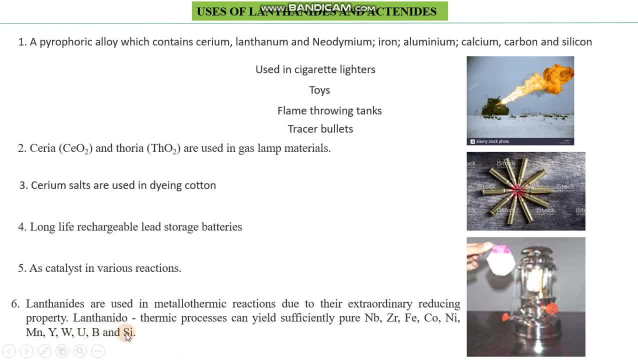 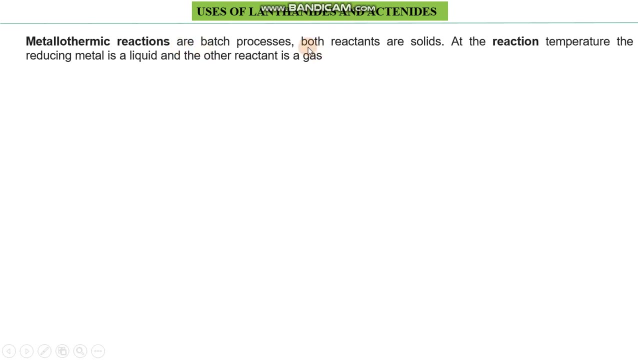 tungsten, uranium, boron and silicon. so, for example, these metals can be used in pure form because of the use of metallothermic reactions. now, what are metallothermic reactions so here? in this case they both the reactants and product. both the reactants are normally in solid states, so it means the metallothermic. 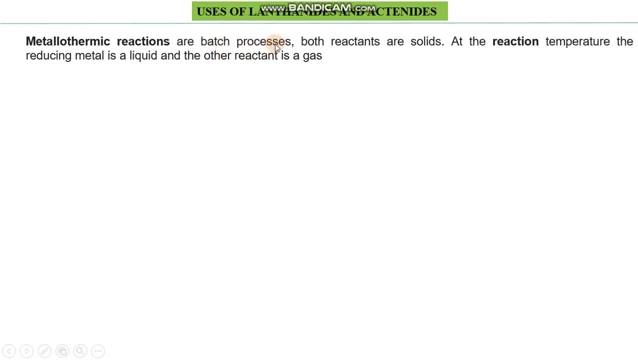 reactions are solid-state reactions and they are used normally, in which process, in after initiation of reaction or after the reaction starts, the one of the reactant becomes liquid and the other one is opted is as gas. now we can say they are actually the products, so the reducing species become liquid. it. 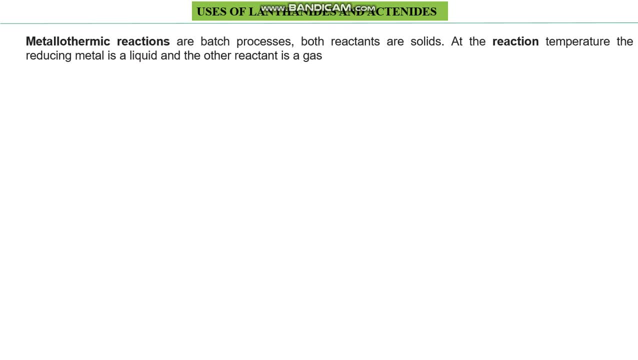 is the reaction temperature and another reactant are. the product becomes gas, so separation of gas from liquid become easy and the liquid, when comes to solid state, it gives the metal and power form. so this reaction, as I told you, can be used for purification of metals are in this reaction. 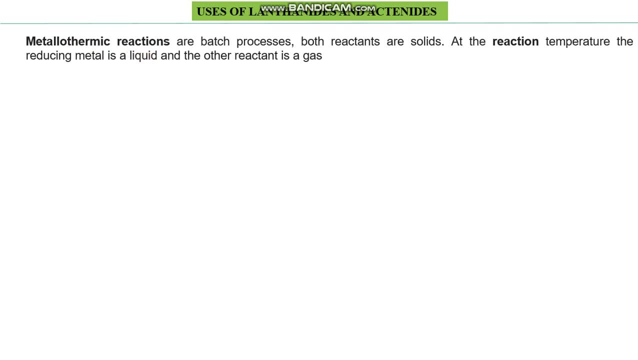 pure metals can be obtained, and the thermal energy produced during this reaction are gaseous. products can be used for further useful purposes. then there are some alloys where the lanthenides and actinides are integral parts of those alloys, and one of the alloys is known as mesh metal, one of the 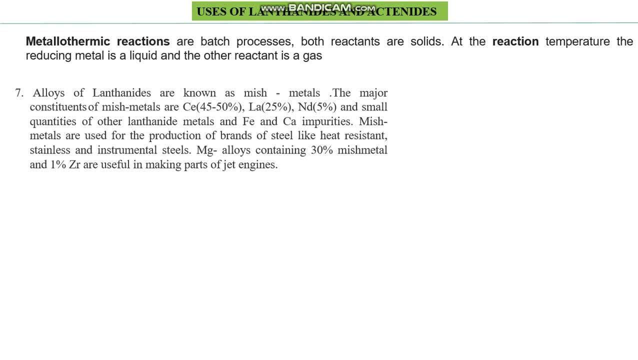 alloy of lanthenides and actinides is known as mesh metals. It is known as mesh materials and this mesh metal contains a major portion of lanthenides, that is, Cerium, lanthanum and neodymium, and these alloys can be useful in the process of reviving. 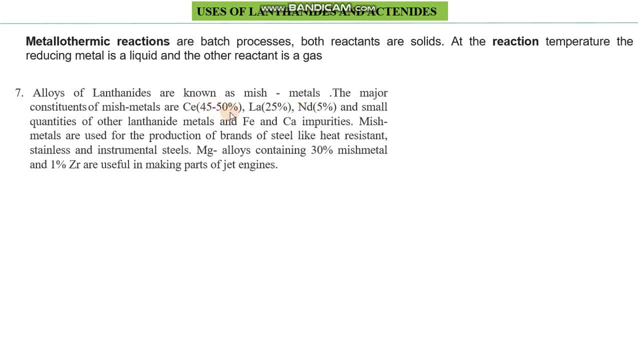 before we particularly go over the actual role of the alloys, very briefly, after fathering down other materials, they can be basically used in therapy asиеes- oh, that is Cerium, lanthanum, and you the aliases that combined in the mold, neodymium. and if you look at the percent, percent amount present in the alloy, so they are. 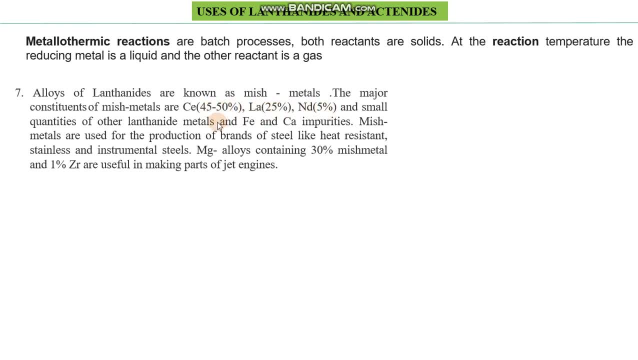 sufficiently, the percentage is sufficiently high, and some small amount of other lanthanides can also be used in this mesh alloy mesh metals, and except lanthanides and actinides, iron and calcium can also be used, which are regarded as impurities. so these mesh metals, they are used for some. 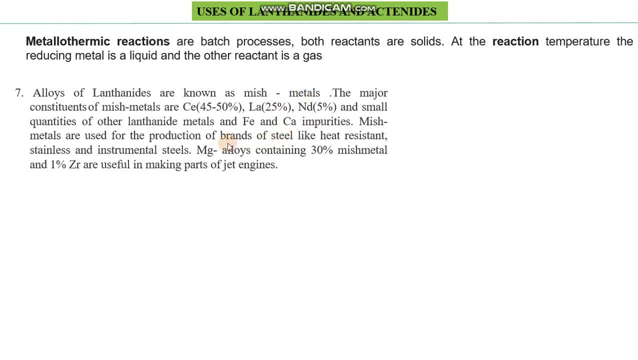 specific purposes, for example, in production of special brands of steel, like heat resistant steel, stainless steel and those which are used in instruments. so they are definitely high quality Steel's and high quality skills are produced because of this. mesh metals- magnesium alloy- in mesh metals containing magnesium up to thirty percent and one percent. 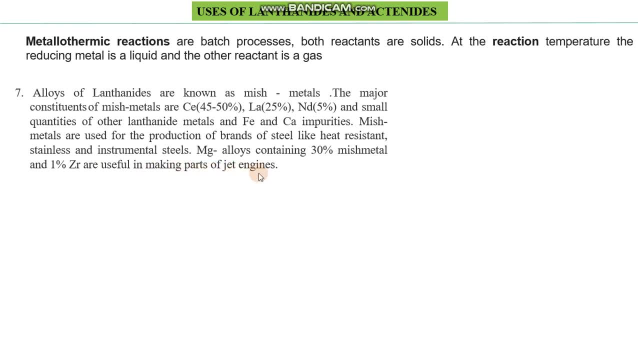 of the metals are mixed with steel and in addition, they get to be used in many products- zirconium. they can also be used in parts of jet engine when they are produced, so this is even more expensive or more useful. alloy of lanthanides and actinides and some non-f block elements. the 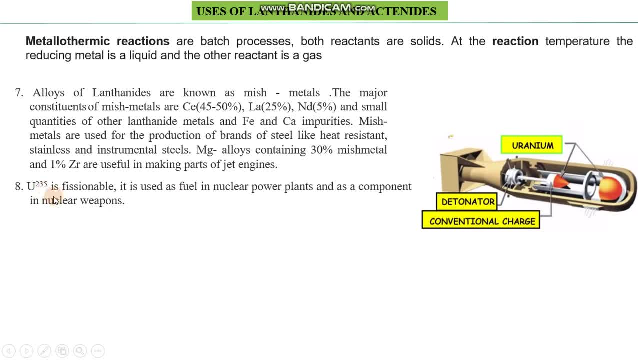 uranium, which is the, which is a member of the actinide series and, if you remember, with atomic number 92, so this is in the beginning of the series. this is fashionable, or it undergoes natural disintegration and is used as fuel in nuclear power plants, so this can also be used.